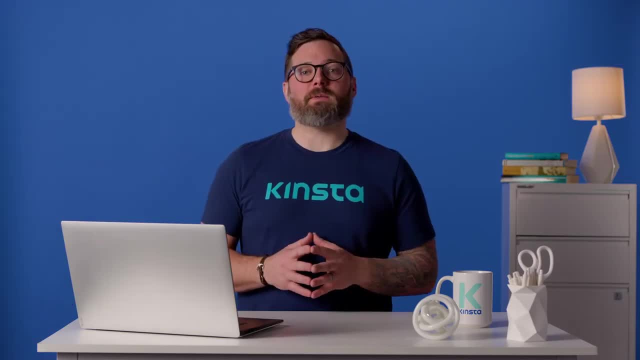 The latest versions of MySQL are better optimized and thus faster. Faster database management software directly translates to lower loading times. However, it may be that you don't know what version of MySQL you're using. If you have full access to your server, you can launch the command line and run the following. 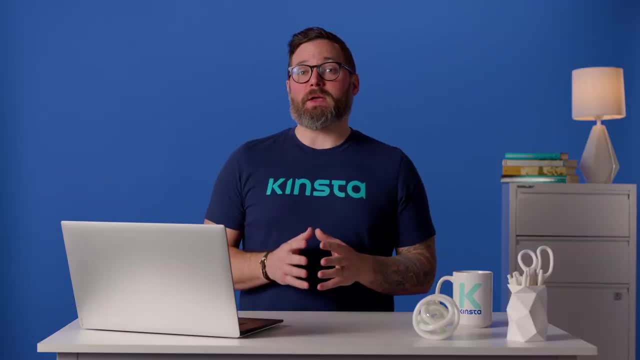 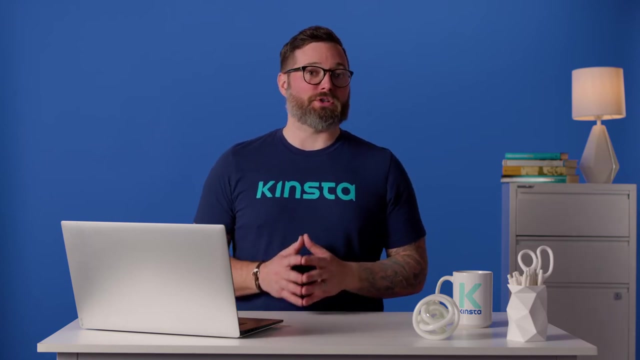 command. The v parameter will return information about the version of MySQL your server uses. You can compare that information against the latest releases on the official MySQL website to see newer versions available. If you're not comfortable using the command line, you can find out what MySQL version you're using through the WordPress dashboard. 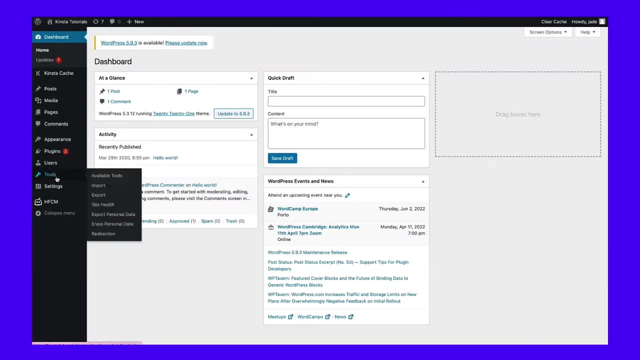 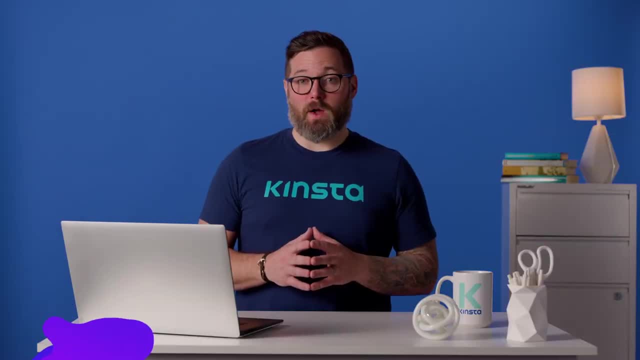 First access the dashboard and go to Tools, and then Site Health. Next, open the Info tab and click on Database. Depending on the version of MySQL, the software might update automatically. If it doesn't, you can use the command line to update MySQL to the latest version. 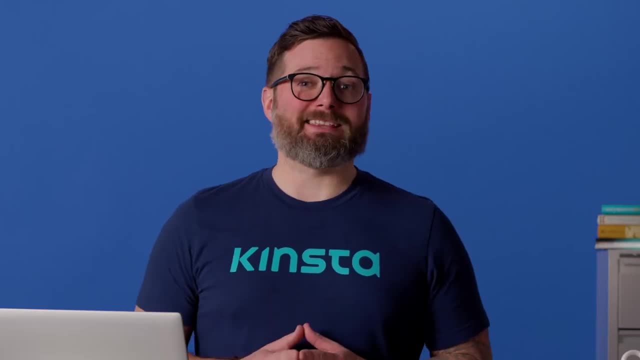 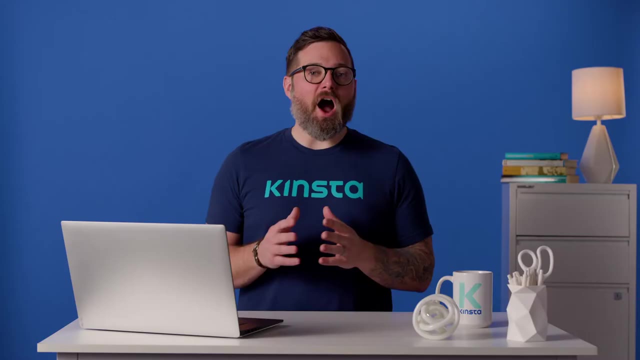 If you're using Kinsta, you don't have to worry about updating the database management software. Instead, we automatically update clients to the latest version, To the latest stable version of MariaDB. Often the plugins and site themes you want to install from your website. 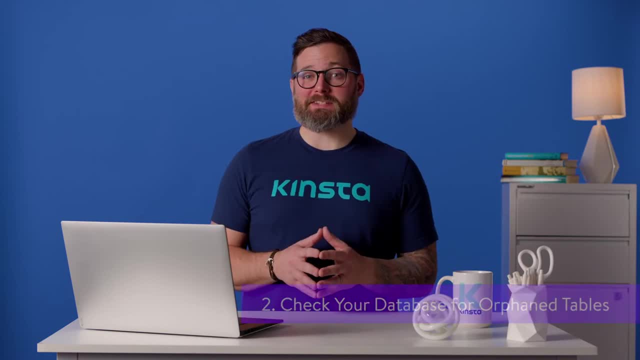 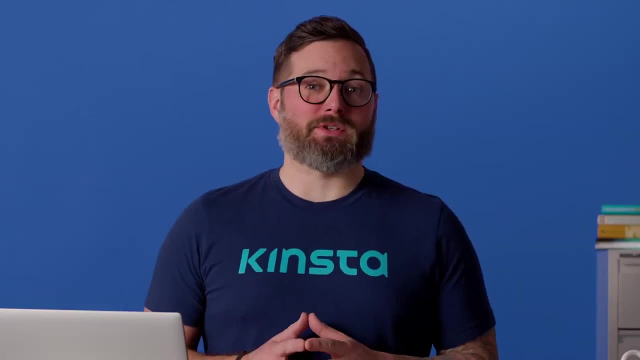 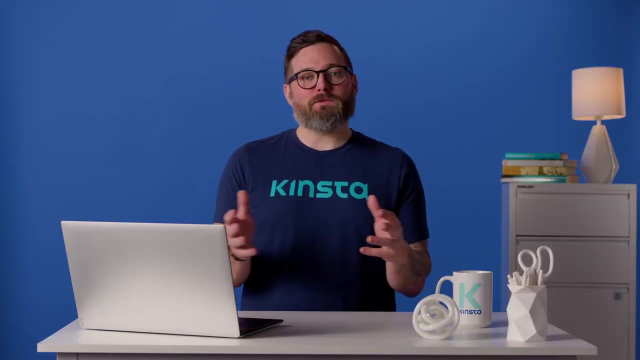 will leave data behind. This can be due to poor coding standards or because the plugins and themes decide to store that data in case you want to reinstall them. The idea behind this approach is that leaving settings and configurations stored in your database will save you time and work down the line. However, all of those unused tables can 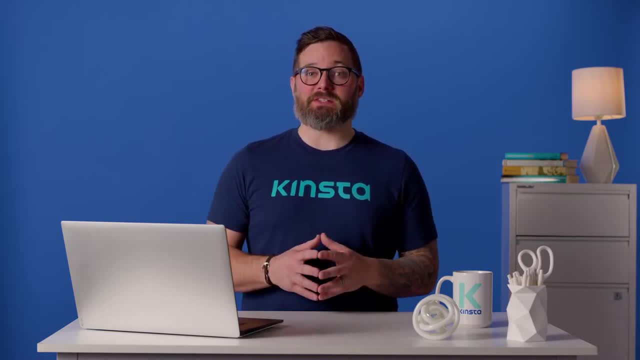 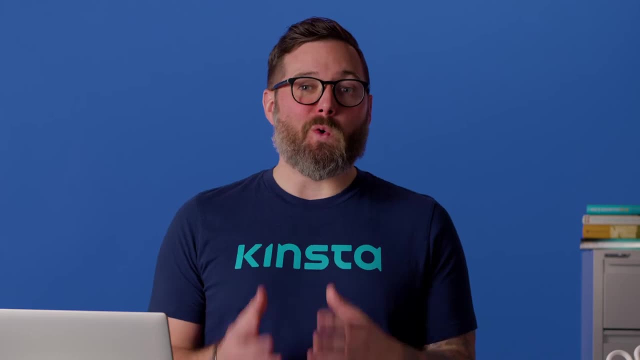 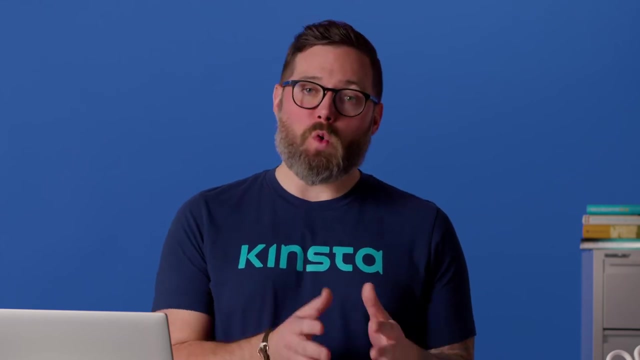 lead to a bloated database, which in turn may slow queries down, depending on your server's capabilities. Ideally, you can clean that up after you uninstall plugins, so you can prevent orphaned tables and data from accumulating. There are two ways you can go about that task: either manually or using a plugin. 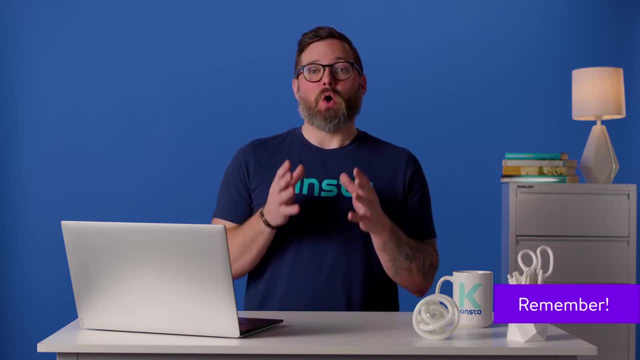 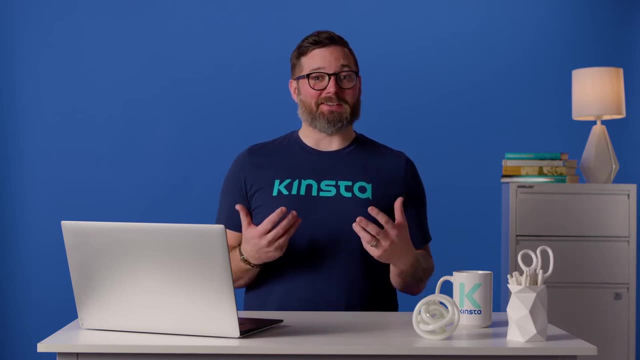 Before you make any changes to your database, in any situation, we recommend that you fully back up your WordPress site. That applies even if your host does daily backups, as Kinsta does, so you'll have a copy of your site to revert to if needed. Once you have a backup, you can access. 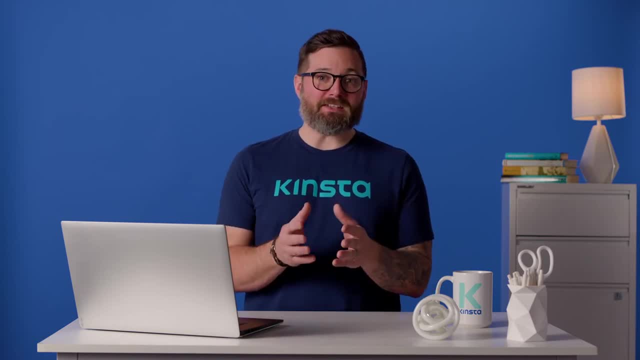 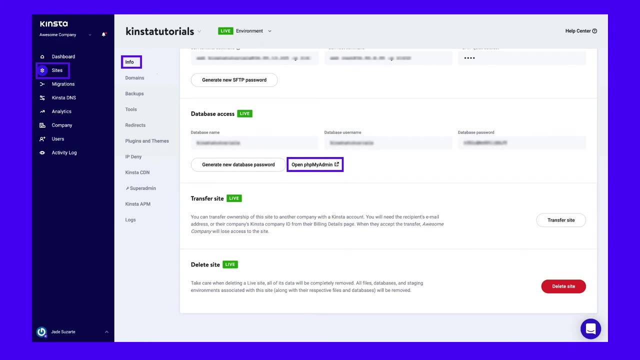 your database via phpMyAdmin. If you're a Kinsta customer, log into your MyKinsta dashboard and go to Sites. Select the site you want to work on and jump to its Info tab. There you'll find a link that will give you a direct access to your database via phpMyAdmin. 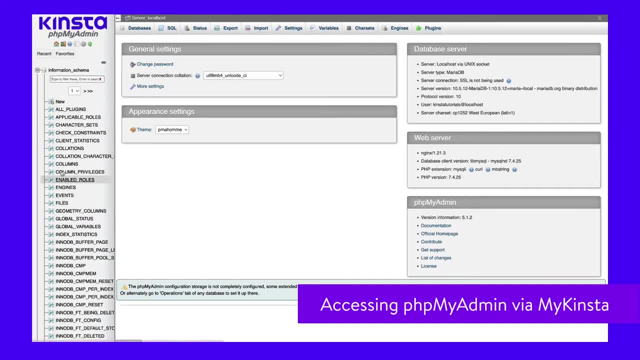 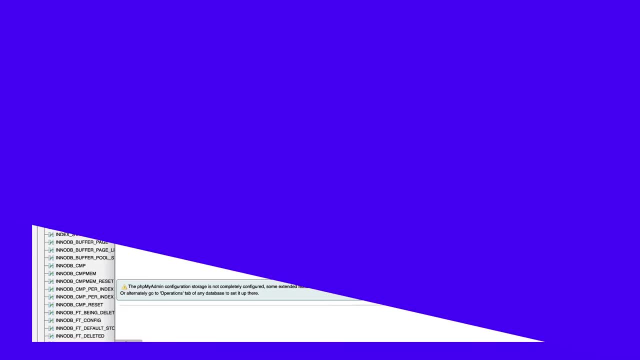 Once you're inside phpMyAdmin, you can use the software's search feature to find orphaned tables related to specific plugins. The issue with this method is that it can be hard to know what queries to use unless they're in your database. If you want to access your database via phpMyAdmin, you can. use the software's search feature to find orphaned tables. The issue with this method is that it can be hard to know what queries to use unless they're in your database. If you want to access your database via phpMyAdmin, you can use the software's search feature to find orphaned tables. 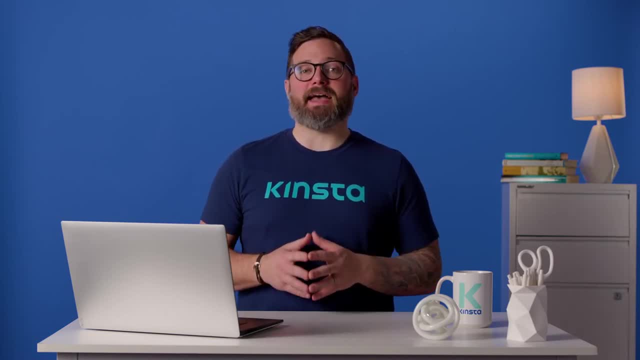 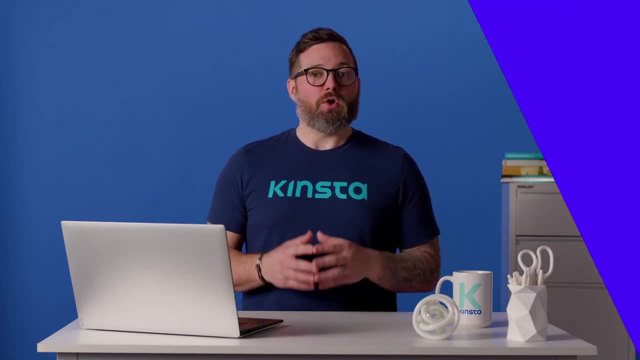 For example, Yoast SEO recommends using the WPSEO query to find tables related to the plugin after uninstalling it. Running a quick search using phpMyAdmin will return a list of entries containing that term across different tables. Although the manual method works, 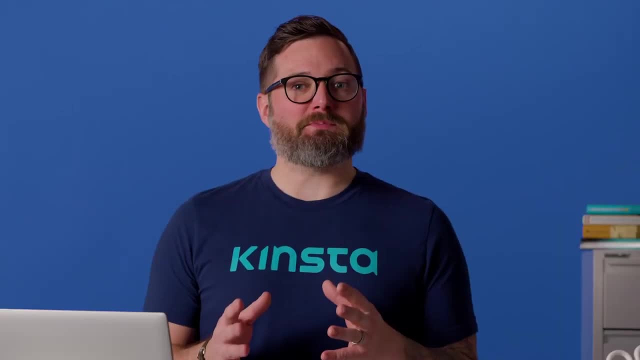 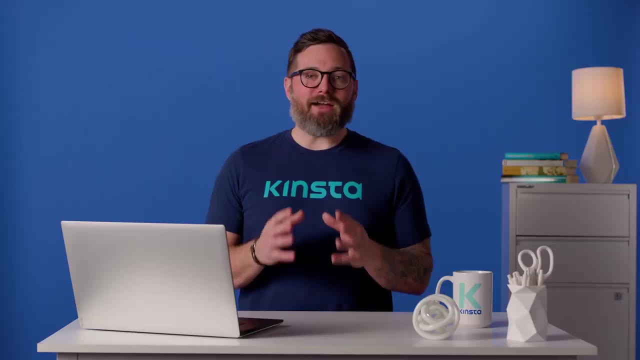 we encourage you to use a database cleaning plugin solution. With some of these plugins, you'll even be able to find orphaned tables from within the dashboard and delete them without having to dig through phpMyAdmin. Every WordPress database includes a broad array of tables. 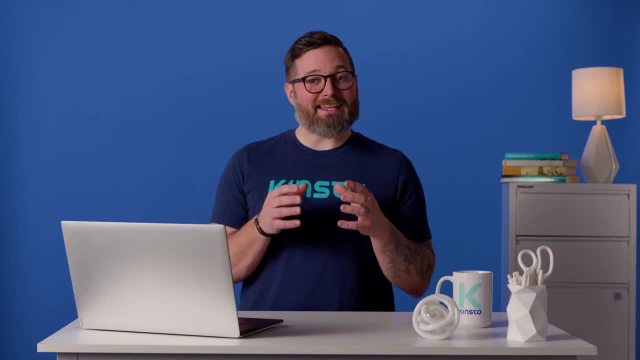 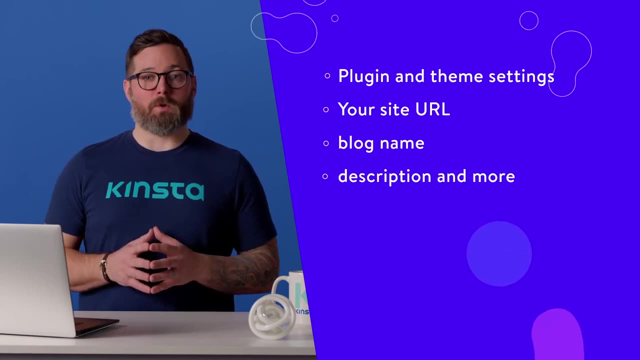 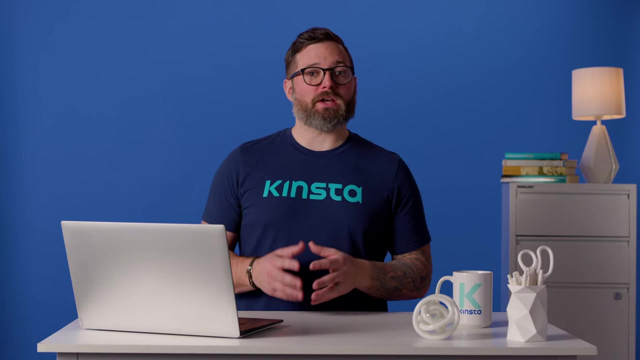 One of those tables is called wp-options and it contains information such as plugin and theme settings, your site URL, blog name description and more. If you check the wp-options table using phpMyAdmin, you'll notice a column named autoload: WordPress checks for rows, with a yes entry under. 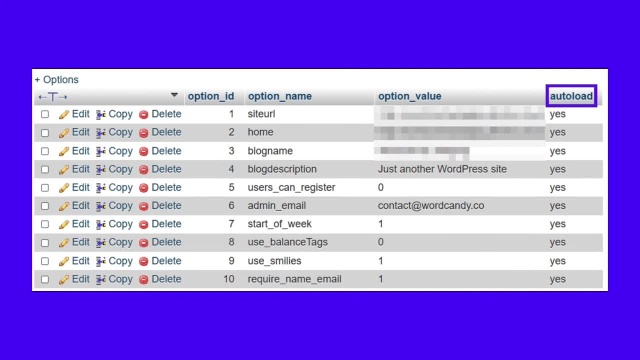 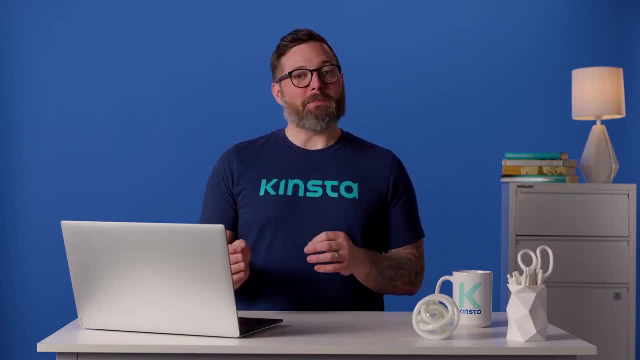 autoload then loads that data every time someone accesses your website and visits any of its pages. Out of the box, WordPress should only autoload critical data. However, some plugins and themes add data to wp-options and configure it to load automatically Over time that autoloading. 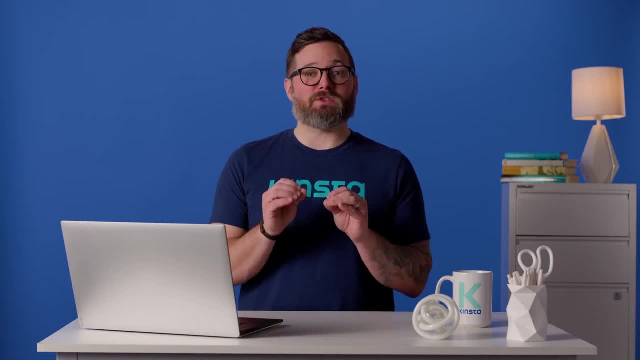 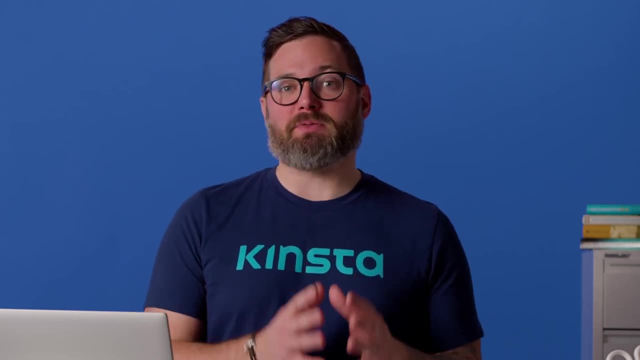 data can slow down response times, just as if you had too many programs set to launch automatically when you turn on your computer. If your WordPress website feels sluggish and you can see many plugin related entries in wp-options, we recommend that you check out how much data autoloads in WordPress. 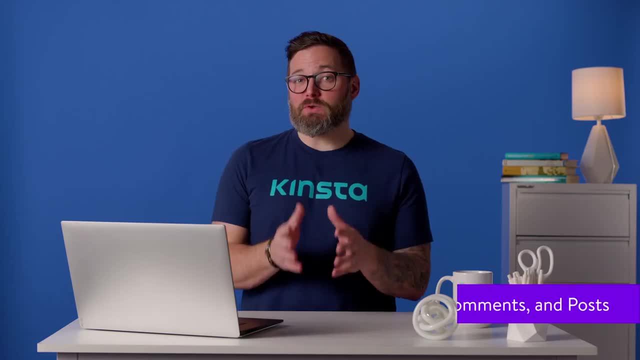 and identify which plugins and themes you should be using. If you're looking for a plugin that's easy to use, we recommend that you check out how many plugins you can afford to disable. As you use WordPress, your website will accumulate a lot of unused data, For example, WordPress. 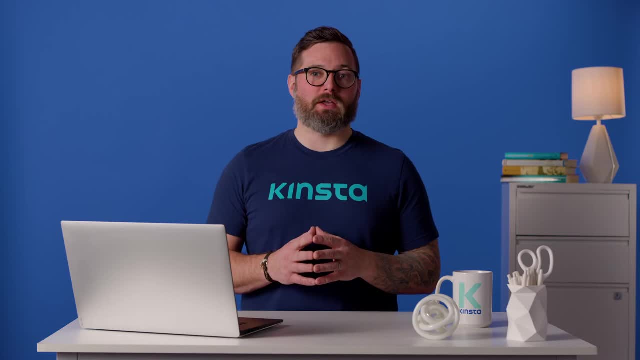 automatically saves several revisions and drafts for your posts, depending on how many changes you make to them Over time. all of the data can bloat your database, so it's good practice to clean up those entries periodically. The best way to do so is with a plugin such as Advanced Database Cleaner.